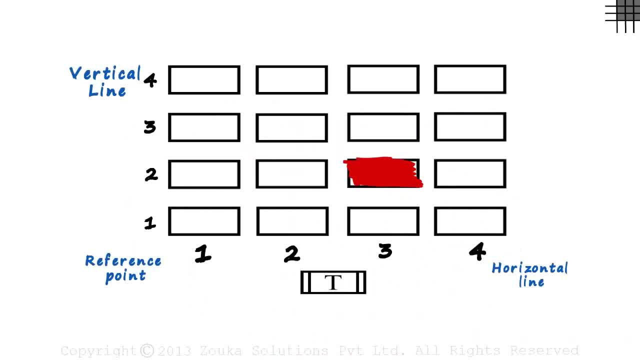 We saw this example in the previous video, where we had to give this bench a unique identity. To give it a unique identity, we needed three things: A reference point, a horizontal line and a vertical line. Let's see how we actually use these three. 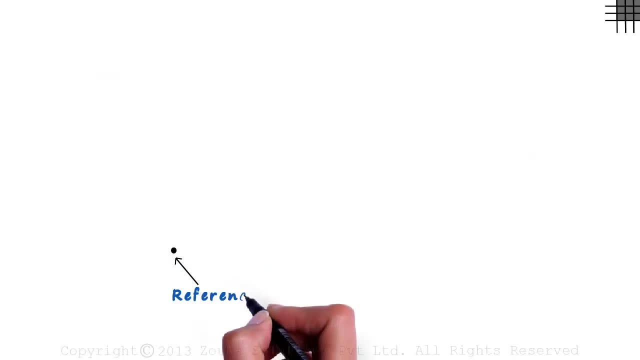 things. Let this be our reference point. We draw a horizontal line from this reference point. Then we draw a vertical line which will be perpendicular to this horizontal line. We will need some numbers to denote the columns. So we mark one, two, three, four and so on in equal intervals. Similarly, on the 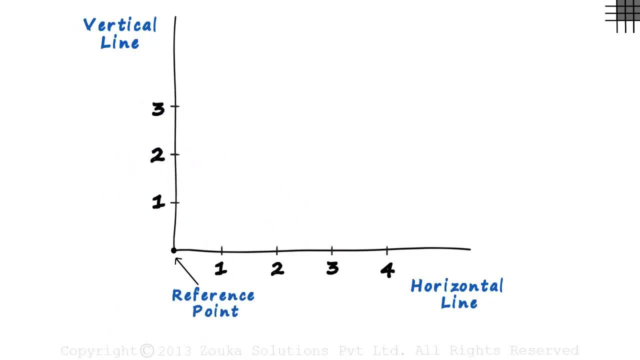 vertical line we mark one, two, three, four, with the same interval length as we had on the horizontal line. There is no limit on the numbers we can mark on the horizontal and the vertical lines, So we mark these arrows at the end of the lines. Most importantly, the reference point will be: 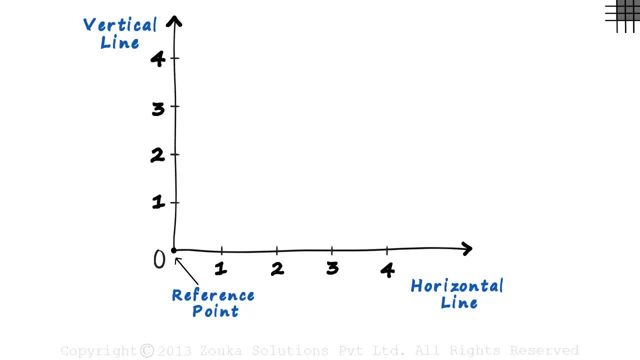 the number zero. Now, if we have any point in the region, we can easily give it an identity based on the numbers we have marked. But wait, What if the point is here? How would you give it an identity? It's simple, We just extend this. 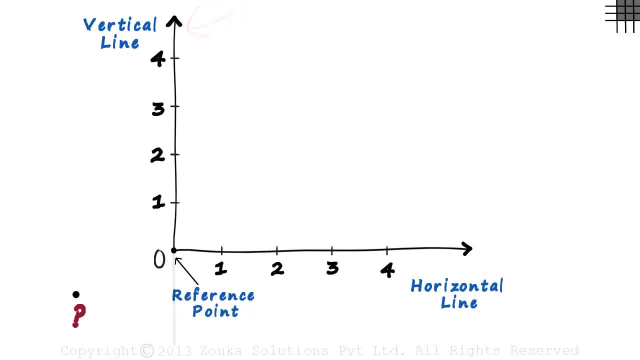 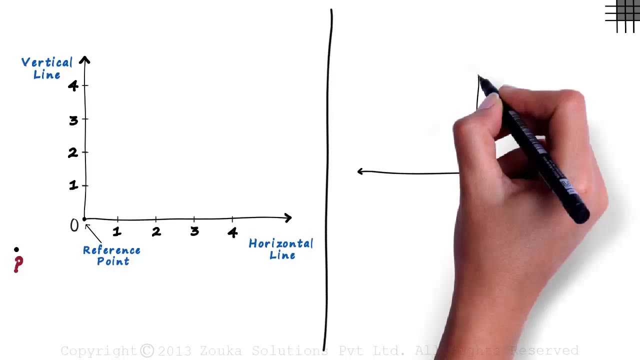 line to the left and this line downwards. Let's zoom out a bit and modify this diagram slightly. We draw the horizontal line like this. Notice that it has arrows on both its ends. The vertical line is drawn like this, again with arrows at: 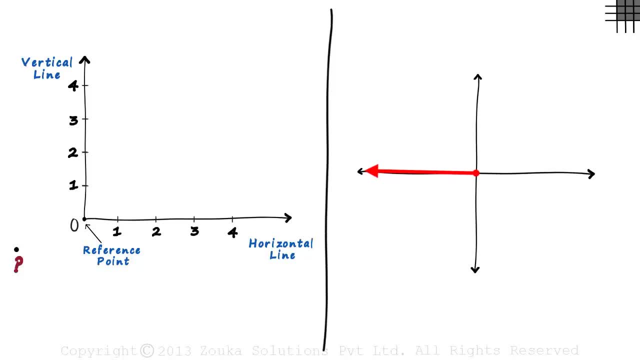 both its ends. We extended the horizontal line to the left and the vertical line downwards. Now, no matter where you place the point on the plane, you will be able to give it a unique identity. We cannot keep calling these lines horizontal and vertical every time. So we name them. We generally call the.